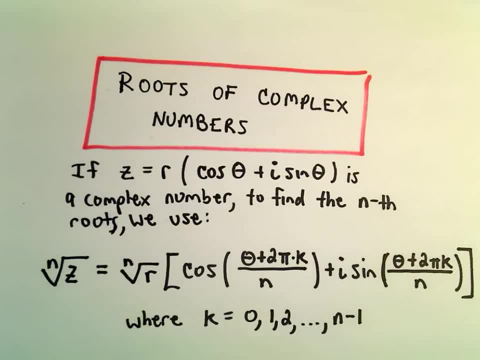 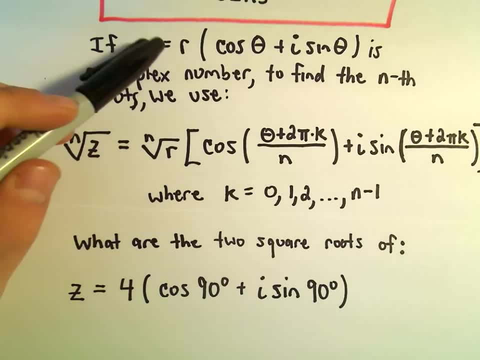 So it looks a little worse than I think what it is, hopefully. So one thing you'll always have to do if you're given a complex number: if it's not already in polar form, you're going to have to put it in polar form. 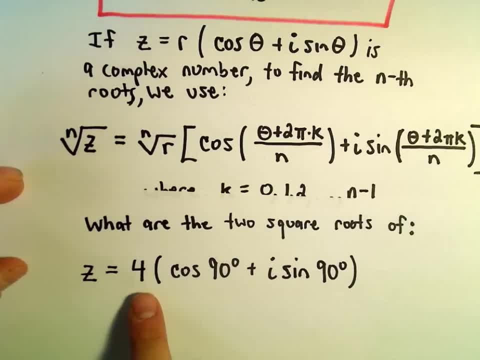 Okay. so in our example here we want to find the two square roots of 4 times cosine of 90 degrees, plus i sine of 90 degrees, And let's just use our formula here. So we're going to take the square roots. 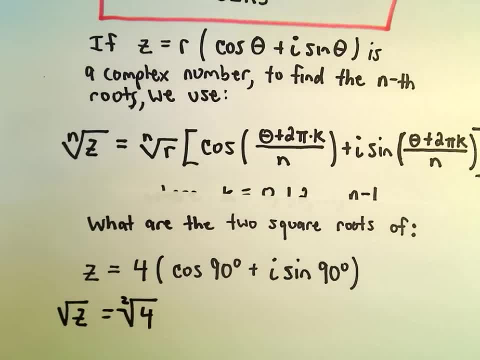 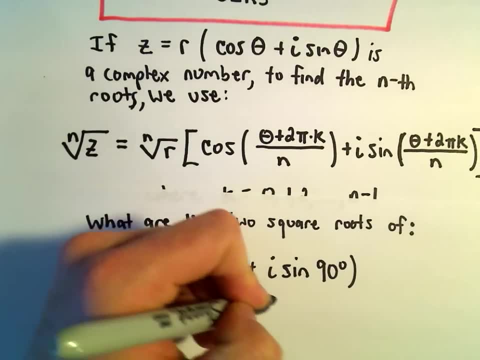 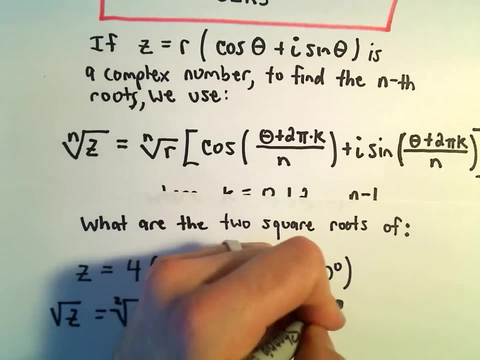 And again, when we're taking a square root, we're taking a second root here. So then we would have cosine of, well, 90 degrees plus. okay, we used 2 pi in the formula. Equivalently, we can use 360 degrees times k. 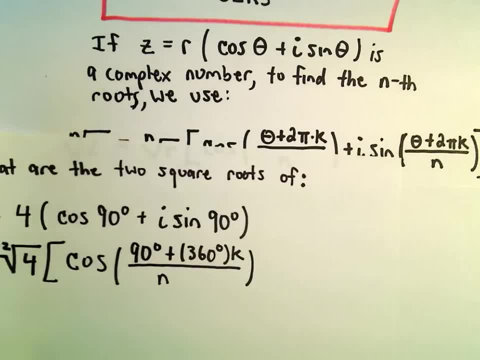 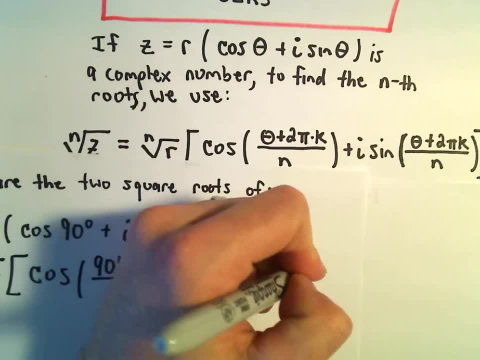 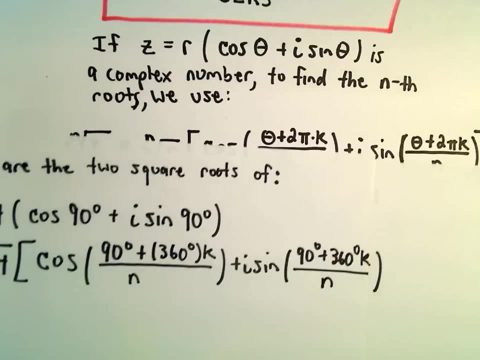 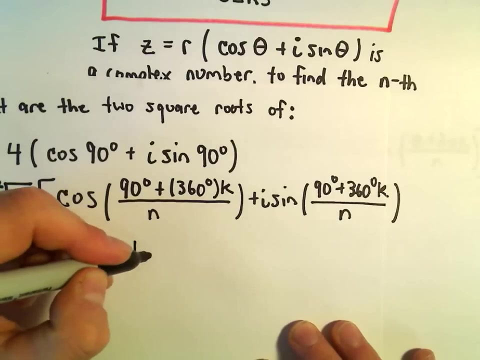 Over n. See if we can't squeeze this one all in here, Plus i sine of 90 degrees plus 360 degrees times k over n. Alright, so now what we have to do? k can vary from 0, 1, up to n minus 1.. 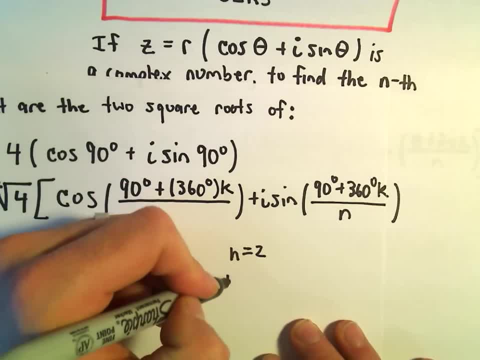 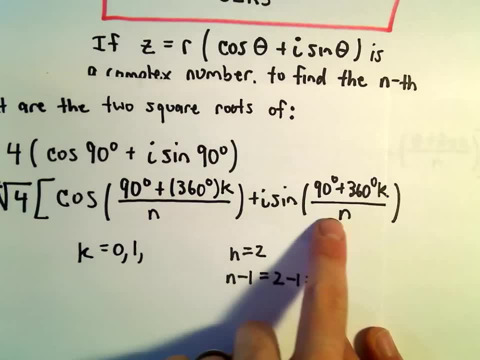 Well, in this case, since n equals 2,, well Well, n minus 1 would be, well, 2 minus 1, or 1.. So the idea is, we're going to have to use this formula, but all we're going to do is we're going to plug in the values: k equals 0 and k equals 1.. 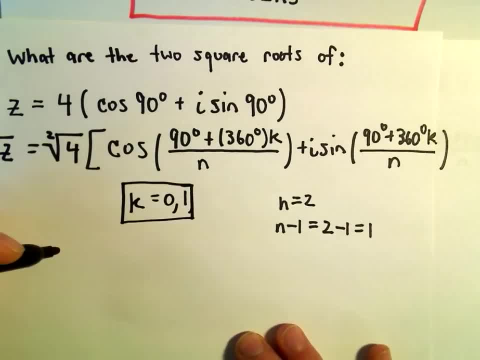 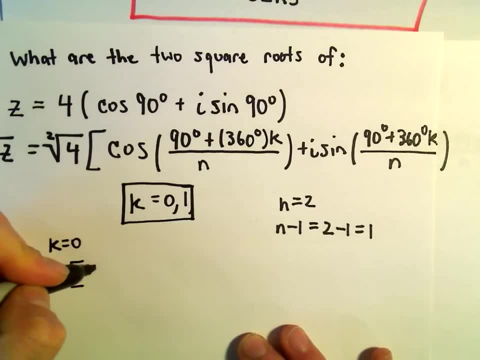 We'll simplify those and those will give us our roots. Okay, so let's do the k equals 0 case. Well, the square root of 4, that's just 2.. And then we would have cosine of, let's see: 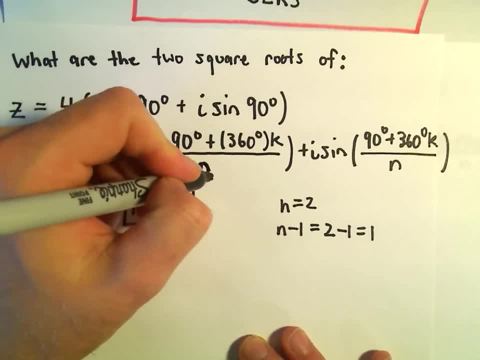 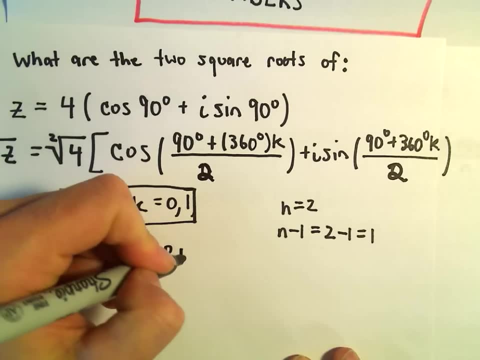 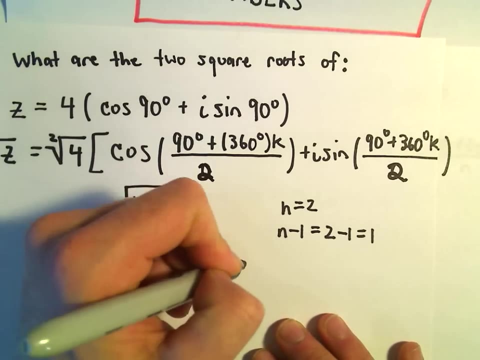 I only put an n in the bottom. We can even go ahead and put the 2 in the bottom in this case. Okay, so we've got 90 degrees plus. well, if we plug in, k equals 0, we'll just get. well, 0 over 2 plus i, sine of, we'll get the same thing. 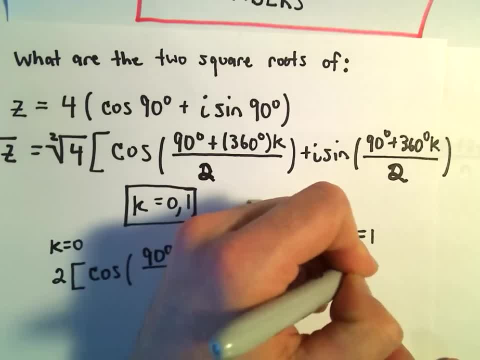 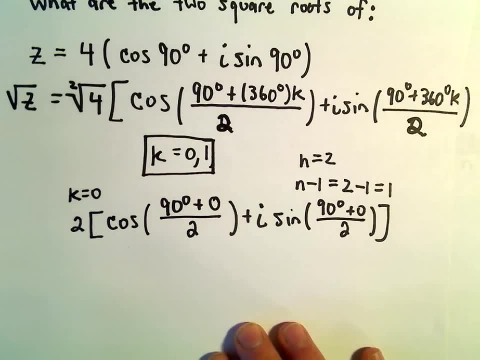 We'll just get 90 degrees plus 0 over 2.. And that's going to be one of our complex numbers. Okay, The other, the other complex number, the root will be when k equals 1.. And if we use k equals 1,, well, again out front, we have the square root of 4,. 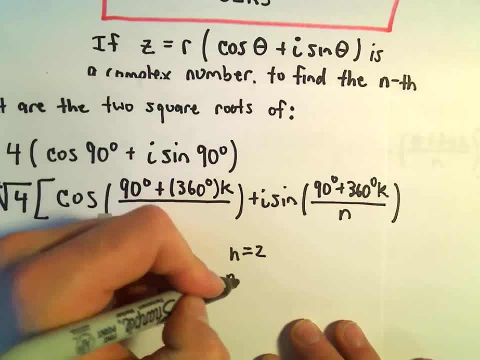 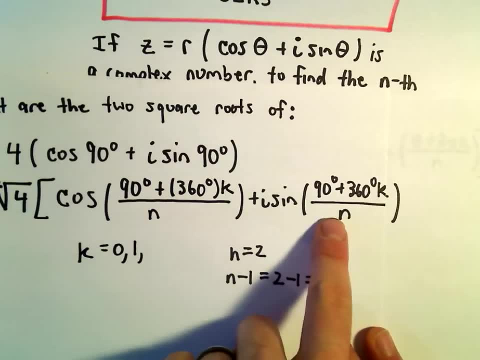 Well, in this case, since n equals 2.. Well, n minus 1 would be: well, 2 minus 1 or 1.. So the idea is, we're going to have to use this formula, But all we're going to do is we're going to plug in the values: k equals 0 and k equals 1.. 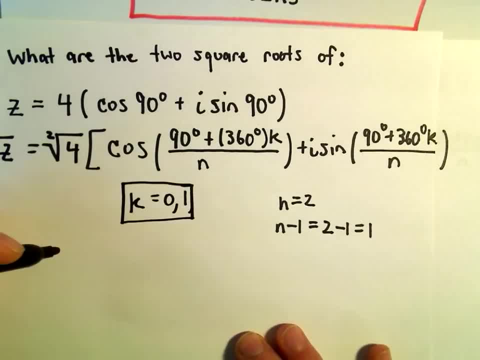 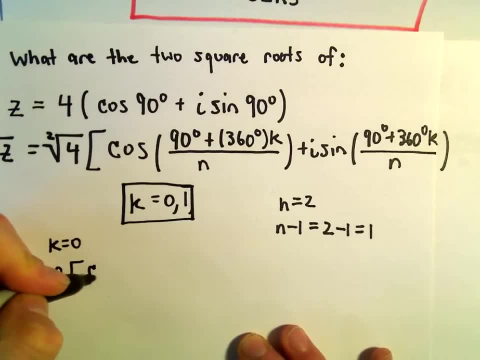 We'll simplify those and those will give us our roots. Okay, so let's do the k equals 0 case. Well, the square root of 4, that's just 2.. And then we would have cosine of, let's see: 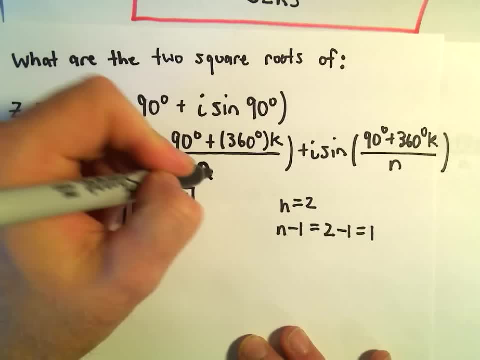 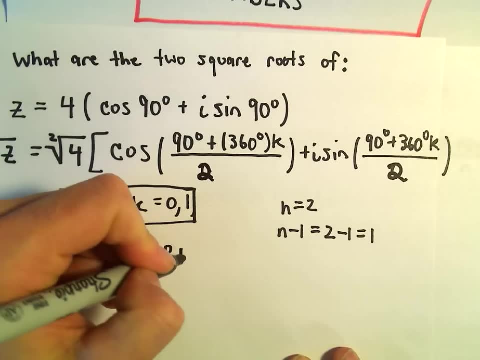 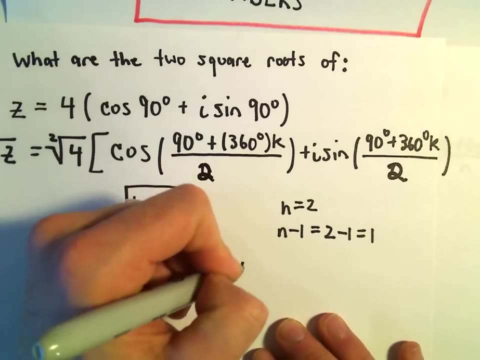 I only put an n in the bottom. We can even go ahead and put the 2 in the bottom in this case. Okay, so we've got 90 degrees plus. well, if we plug in, k equals 0, we'll just get. well, 0 over 2 plus i, sine of, we'll get the same thing. 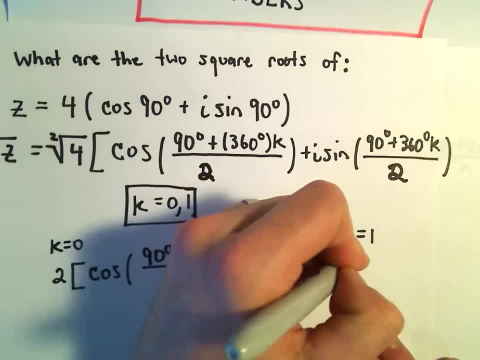 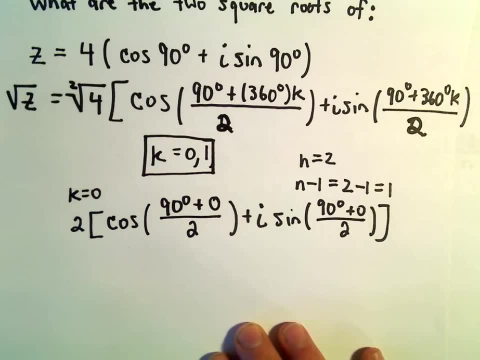 We'll just get 90 degrees plus 0 over 2.. And that's going to be one of our complex numbers. The other complex number, the root, will be when k equals 1.. And if we use k equals 1,, well, again out front we have the square root of 4, which is just going to give us 2.. 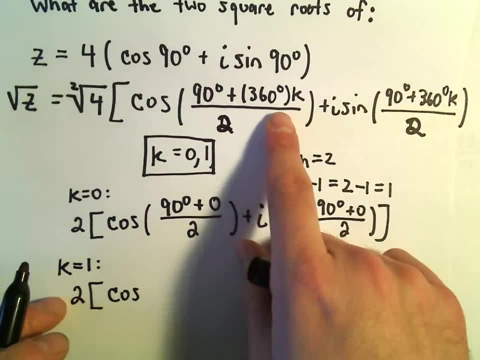 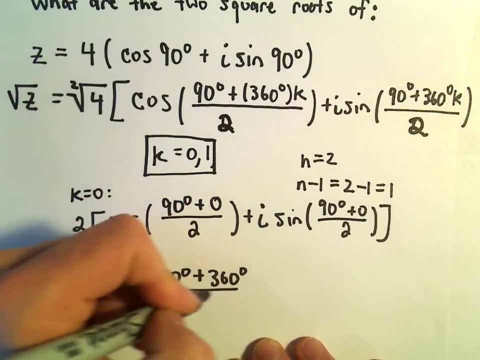 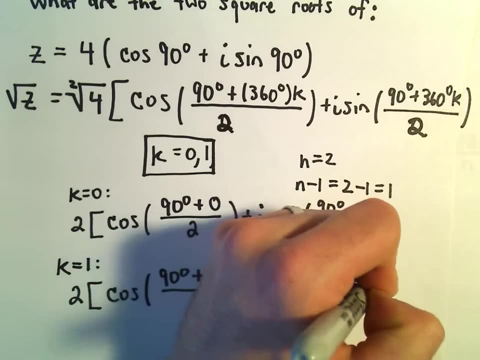 And then again just plugging in k equals 1 into our formula, So we would have cosine of 90 degrees plus 360 degrees over 2, plus i sine, So we would have cosine of 90 degrees plus 360 degrees over 2.. 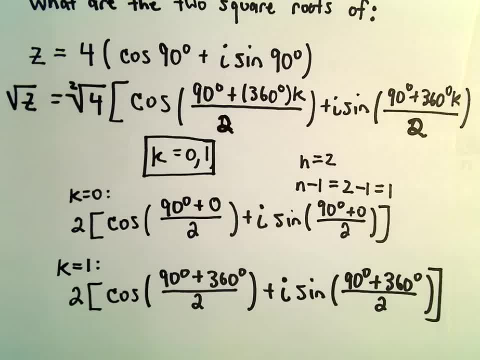 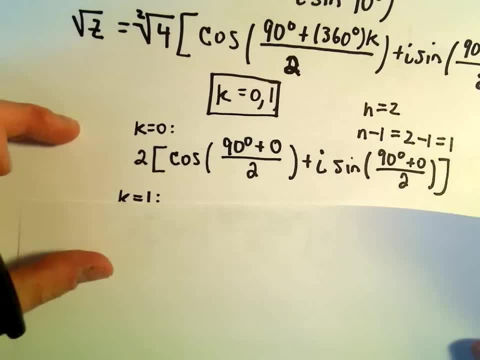 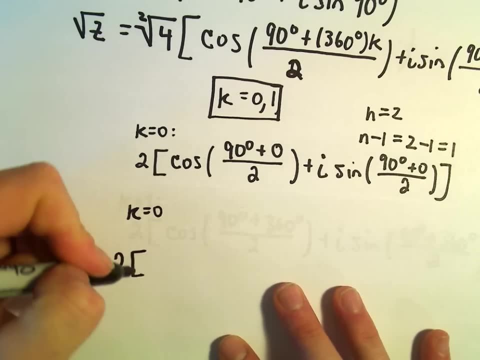 And that would be the other one. So let's go ahead and simplify these down a little bit. So let's see We've got. so for our k equals 0 case, we've got 2 times cosine of. well, 90 degrees over 2 would give us 4.. 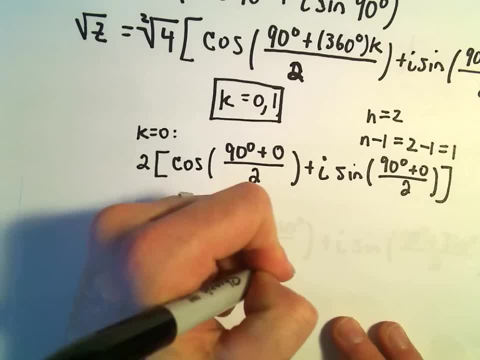 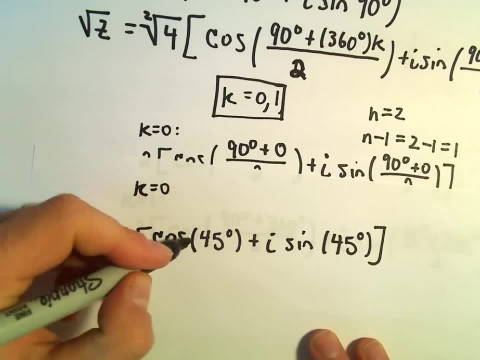 So that's 45 degrees, plus i sine of the same thing, which will be 45 degrees, And again we can always clean this up a little bit. Cosine of 45 degrees, that's root 2 over 2.. 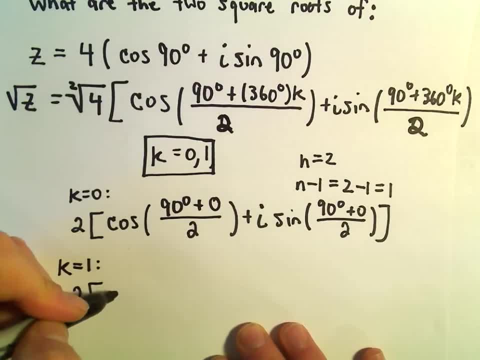 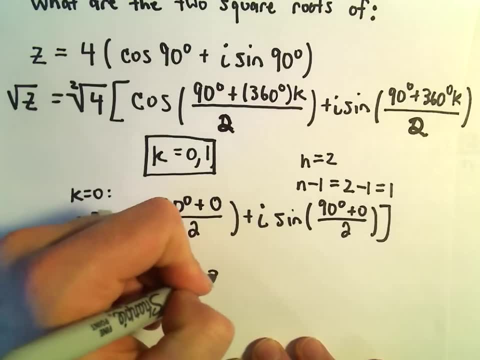 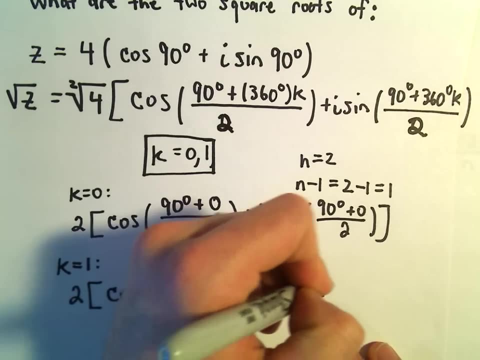 which is just going to give us 2.. And then again just plugging in k equals 1 into our formula, So we would have cosine of 90 degrees plus 360 degrees over 2 plus i sine of 90 degrees. 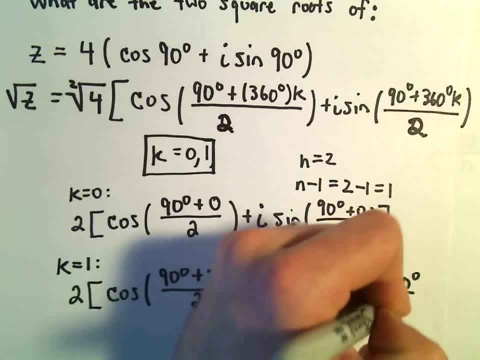 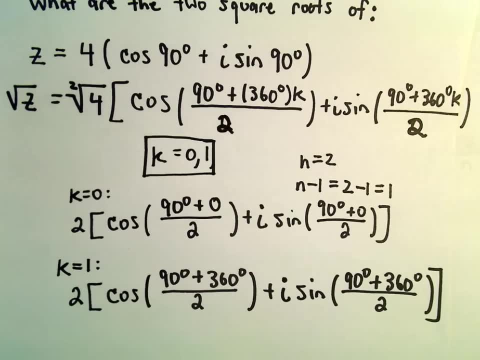 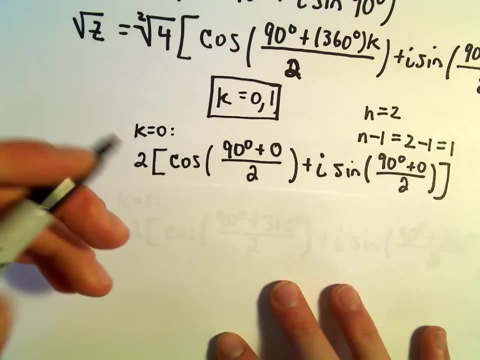 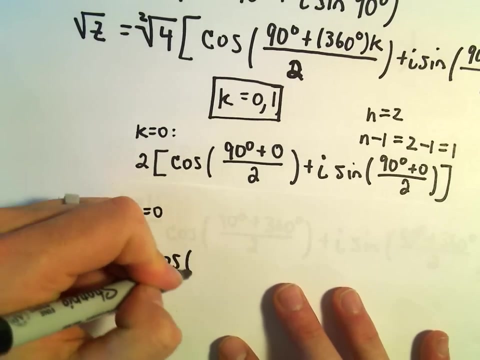 Plus 360 degrees over 2.. And that would be the other one. So let's go ahead and simplify these down a little bit. So let's see We've got. so for our k equals 0 case, we've got 2 times cosine of. well, 90 degrees over 2 would give us 45 degrees. 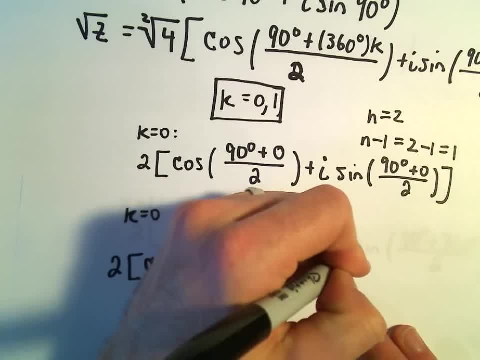 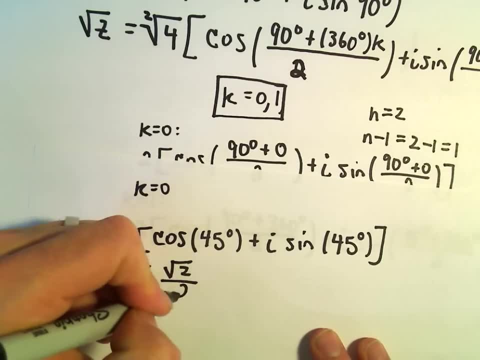 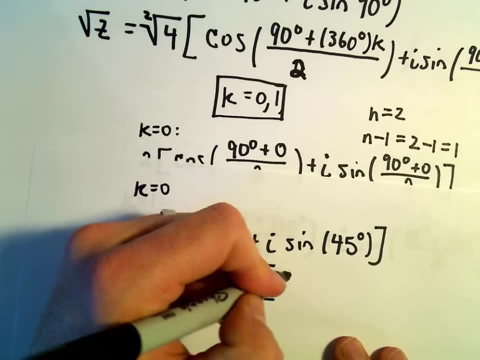 Plus, i sine of the same thing, which will be 45 degrees, And again we can always clean this up a little bit: Cosine of 45 degrees, that's root 2 over 2.. Sine of 45 degrees is also going to give us square root of 2 over 2.. 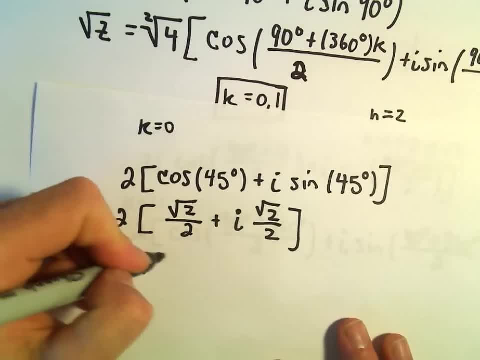 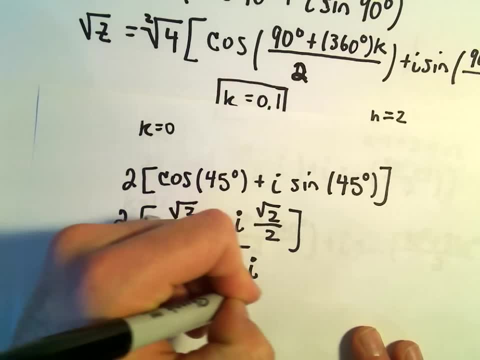 And if we distribute out the 2, the 2s will cancel And we'll just be left with the square root of 2 plus the square root of 2i. Okay, so that's going to be one of our roots. 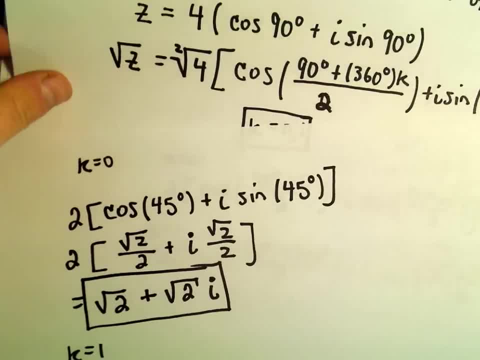 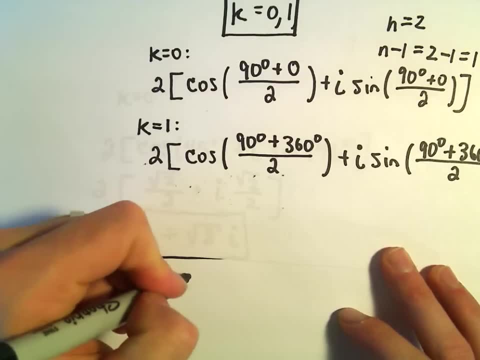 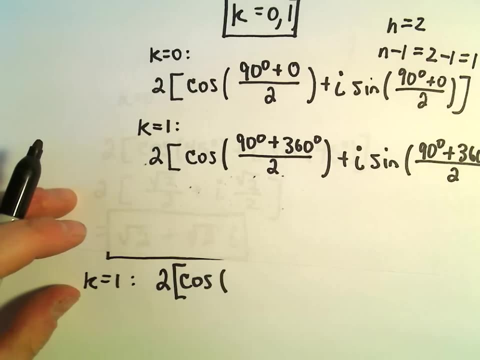 And the other will be when k equals 1.. Let's see So: when k equals 1, this was our other value. So when k equals 1, we'll get 2 times cosine. Let's see So: 90 plus 360, that's going to be 450. 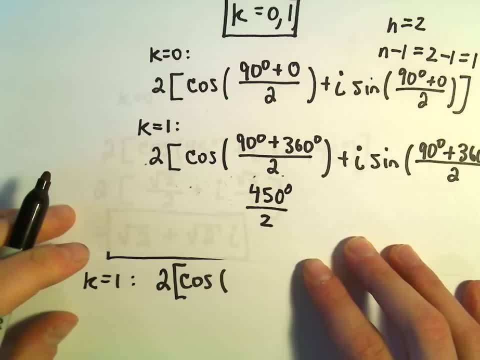 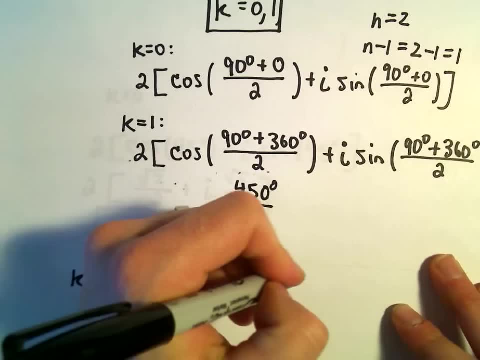 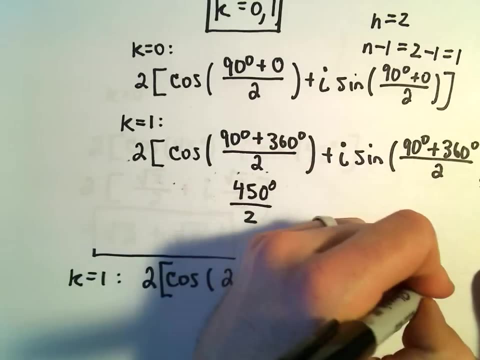 So we'll have 450 degrees divided by 2.. Well, 450 degrees divided by 2. It's going to give us 225 degrees Plus i sine of the same thing, 225 degrees. And now we can always just simplify this down a little bit. 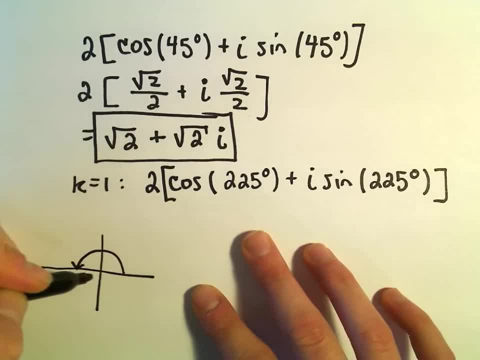 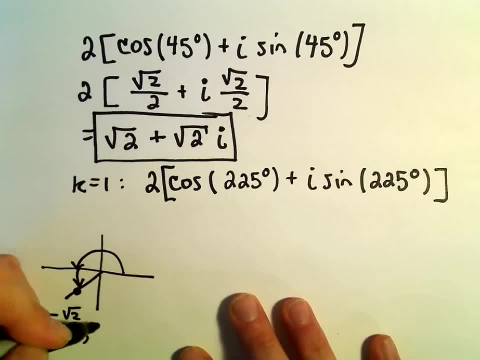 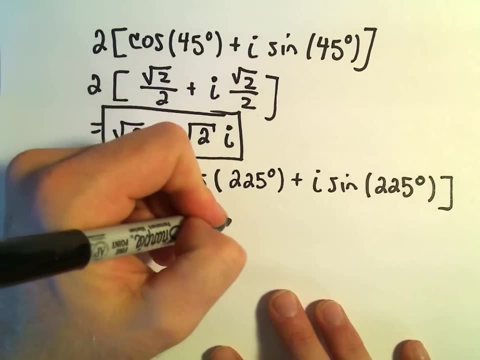 So 225 degrees 180 will be at pi Another 225. At 225, we'll get negative root 2 over 2. Negative root 2 over 2. For both cosine and sine. So we've got 2 times negative root 2 over 2..